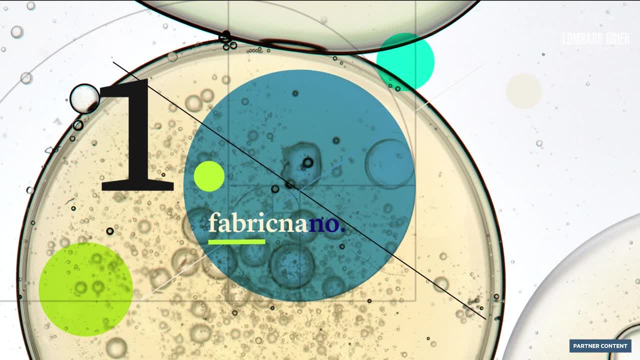 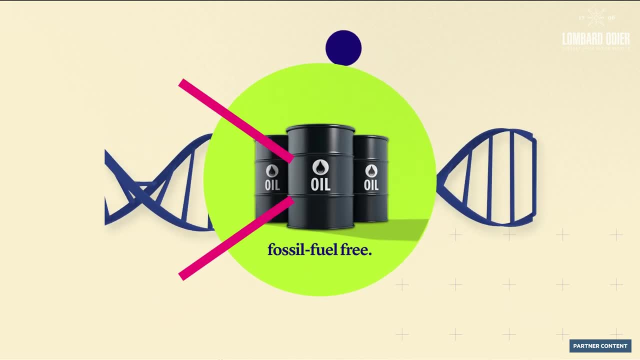 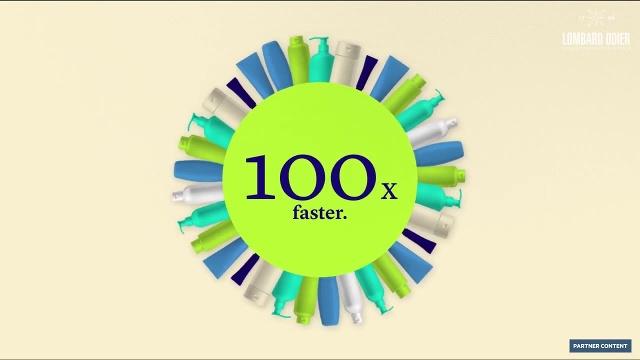 is being done. Fabric Nano is a biotech startup who has found a way to sustainably synthesize bioplastics and fossil-fuel-free chemical ingredients at scale, And produce those chemicals 100 times faster than normal petroleum-based products. Their breakthroughs could mean that 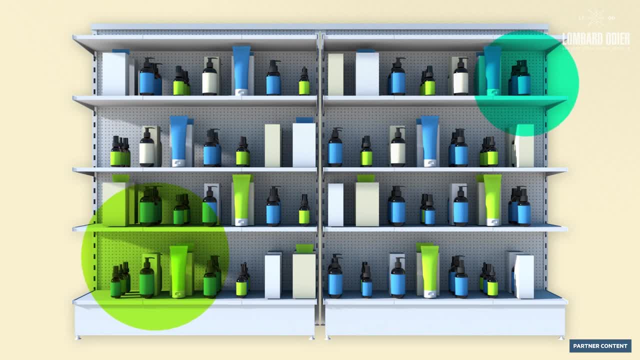 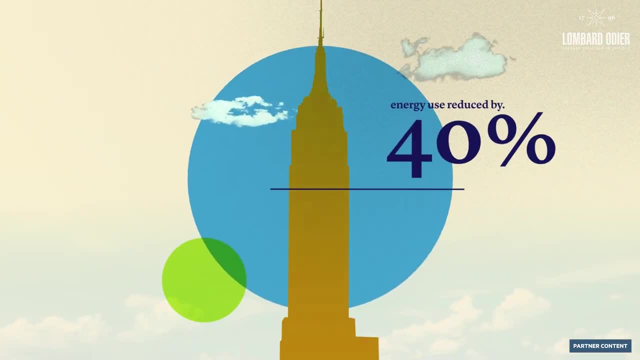 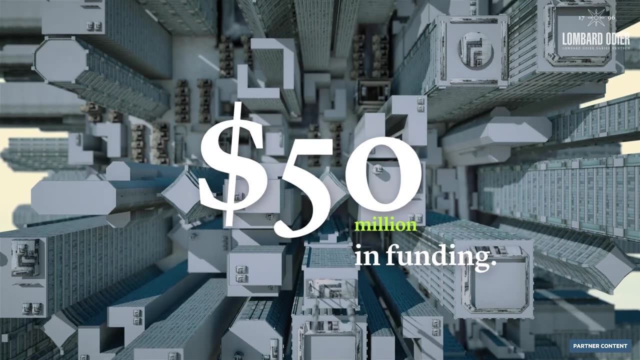 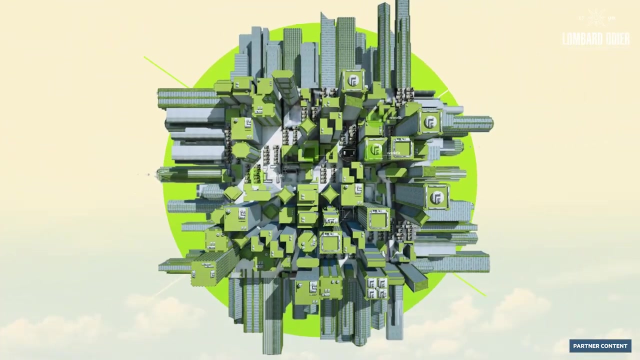 cell-free manufacturing could finally transcend niche to become commonplace. After a hugely successful retrofit of the Empire State Building in New York City, a program called the Empire Building Challenge is providing $50 million in funding to high-rise building owners to pilot innovative retrofit solutions. Although new buildings are easy to make green, old, 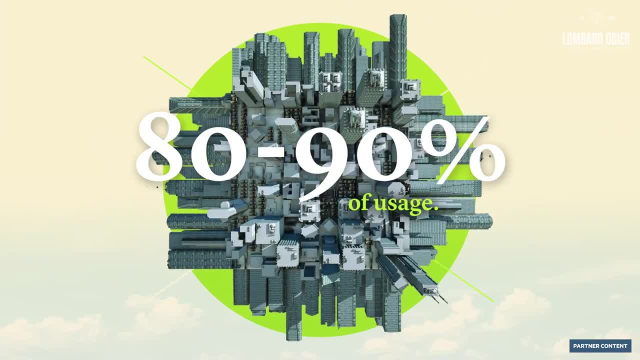 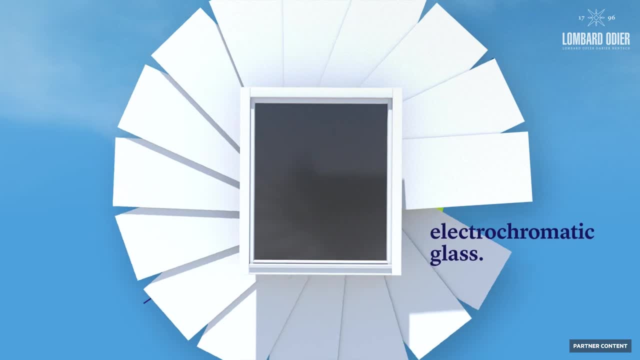 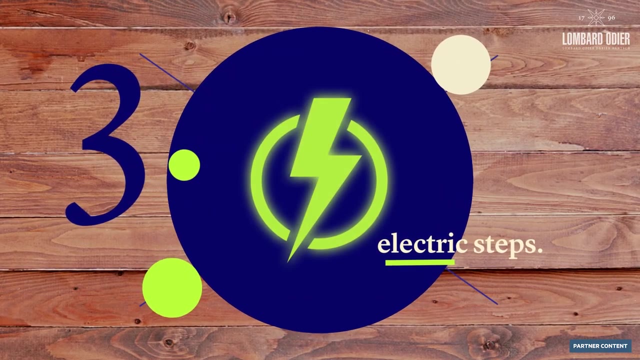 ones make up 80-90% of our usage, And this is where we need to make sustainability gains. The best solutions will be shared widely with other building owners across New York State to create a network of sustainable practice. Making electricity from human-powered steps is a concept that has been around for a while. 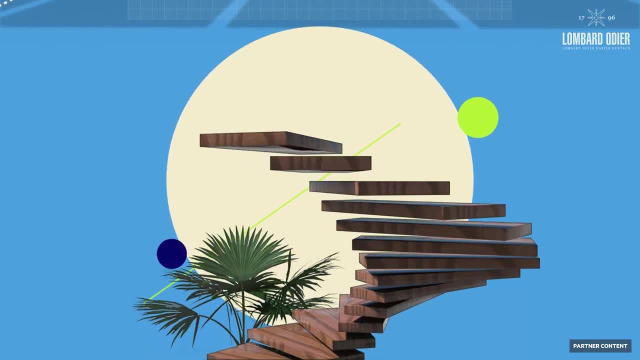 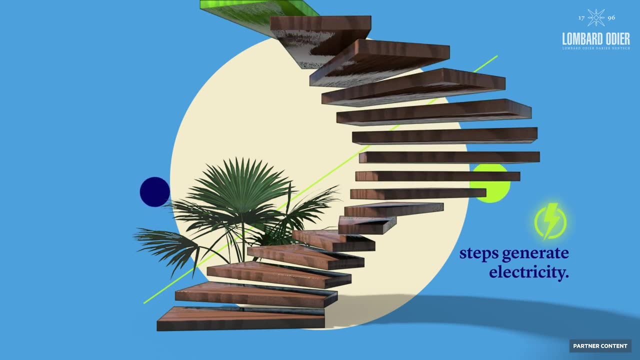 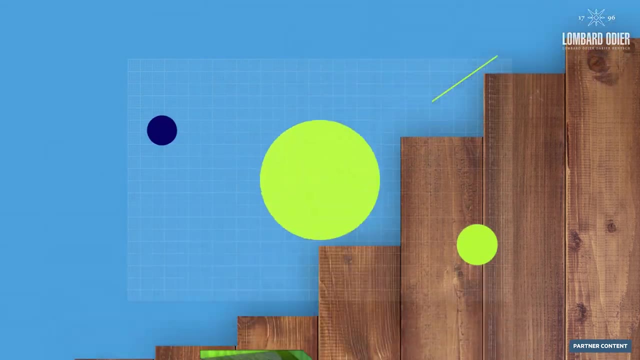 but without a lot of market uptake. But new technology developed by two Swiss labs means that for the first time, we can create electricity from wooden flooring. Wood is one of the most sustainable and popular building materials, But its electro-neutrality has meant that it has been relatively ignored for energy harvesting. These scientists found 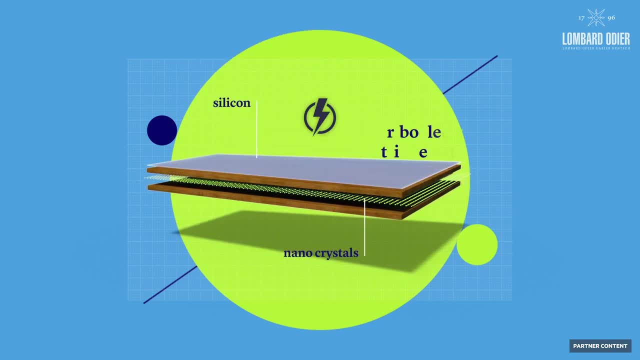 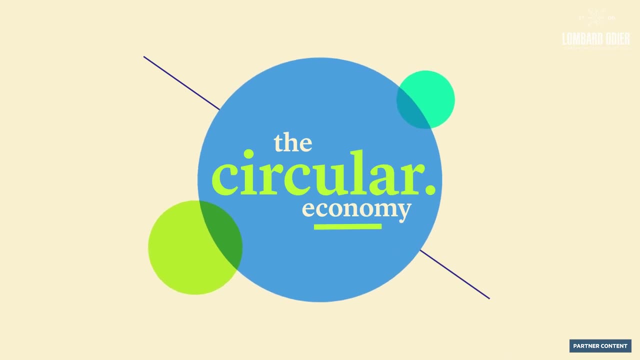 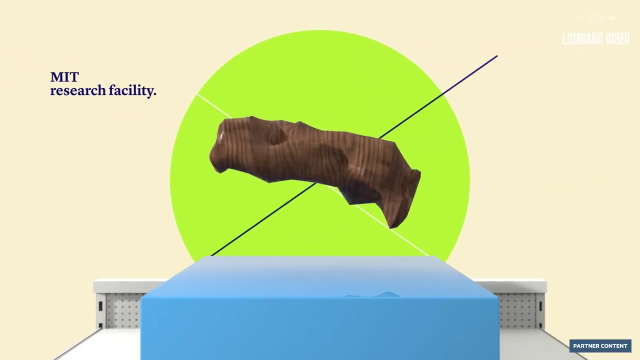 a way to modify it with silicon and nanocrystals – relatively environmentally friendly procedures – making it triboelectric. What if you could grow wood in a lab? Researchers at MIT have not only discovered how to replicate wood by isolating tunable plant tissues, but also to grow it in the lab. The two blue baleen plants are known for their magnificent energy harvesting activities. The research is disappearing when scientists are working on the research to see whether or not they can replicate wood in the natural environment. So it's time to discuss the topic of wood. What if you could grow wood in a lab? Researchers at MIT have not only discovered how to replicate wood by isolating, 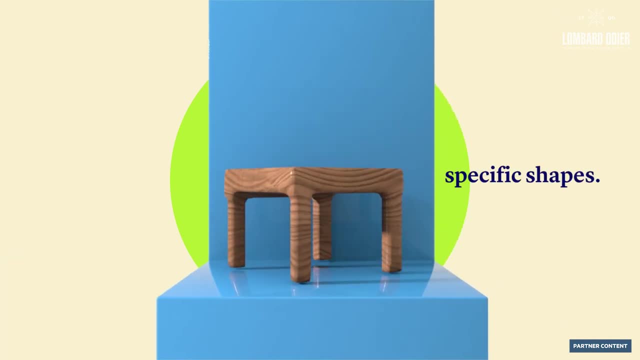 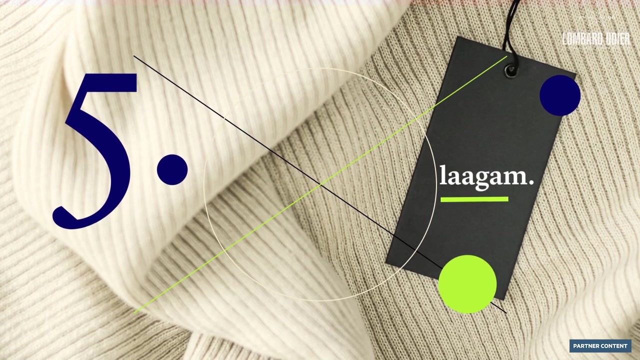 also to grow it in specific shapes, thereby reducing waste, Even though wood can be grown sustainably. this new technology has the capacity to transform our use of biomaterials and combat deforestation. Making affordable fashion sustainable is the goal of this global e-commerce brand. 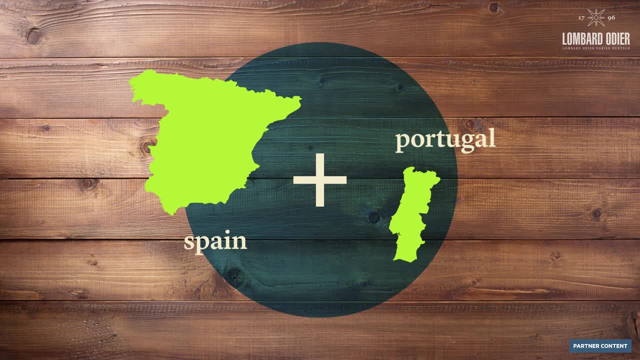 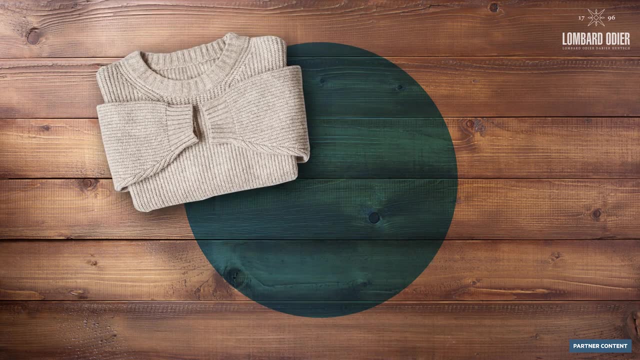 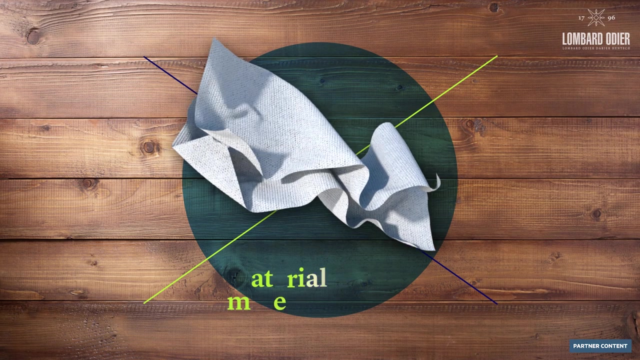 Everything is handmade to order in Spain and Portugal. Most importantly, they only make what is ordered, totally reducing unsold production waste. For every item ordered, they encourage you to resell something you no longer want. They also offset their carbon footprint and donate material scraps to independent fashion. 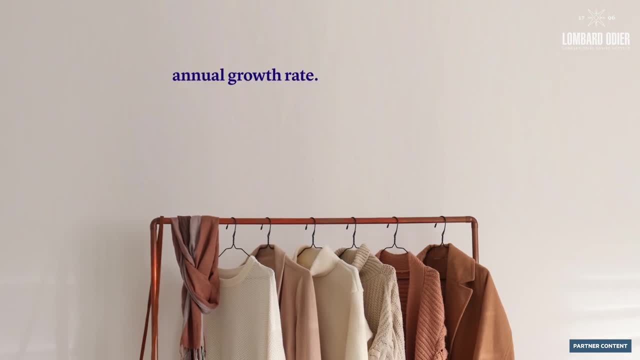 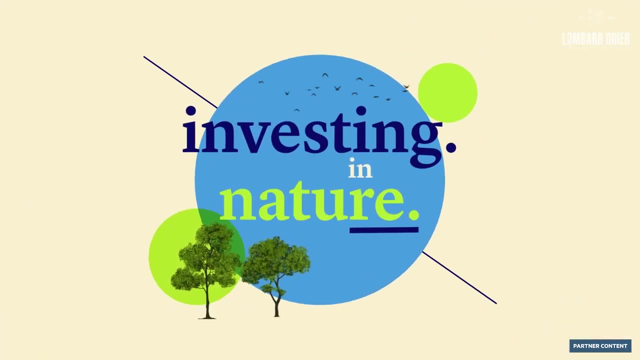 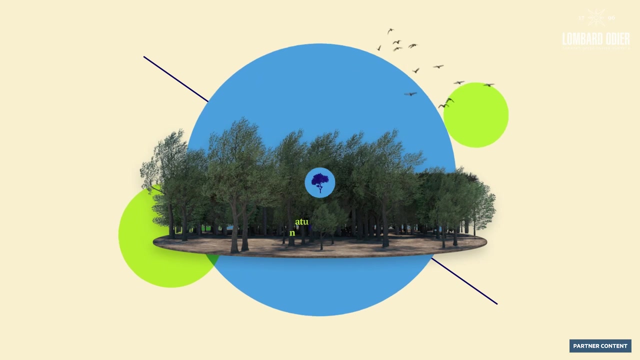 brands, With an annual average growth rate of 100%. this pioneering stockless fashion brand is on the rise, Buying up carbon credits to satisfy sustainability goals. This is not going to fully get us to net-zero. Nature-positive business solutions require that a price be put on negative externalities. 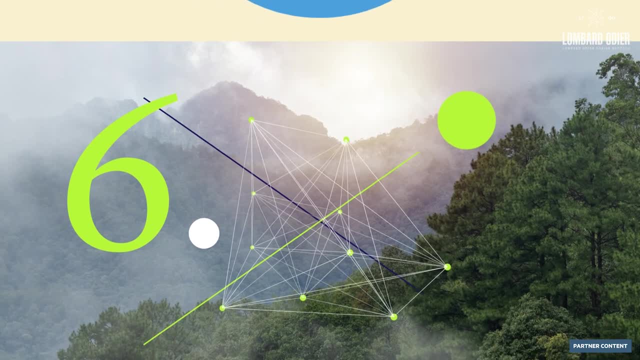 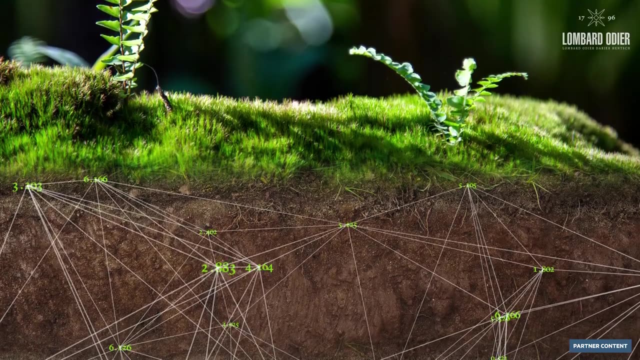 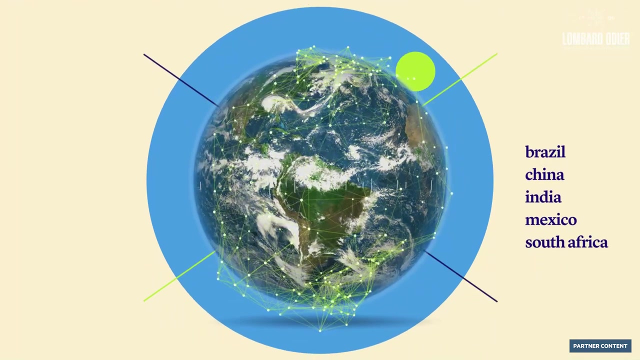 And two companies are helping to do just that. Encaves is a UN-funded research project that is laying the groundwork for environmental and ecosystem accounting, With pilots in Brazil, China, India, Mexico and South Africa. the project is developing the tools, language and structure necessary to achieve this goal. 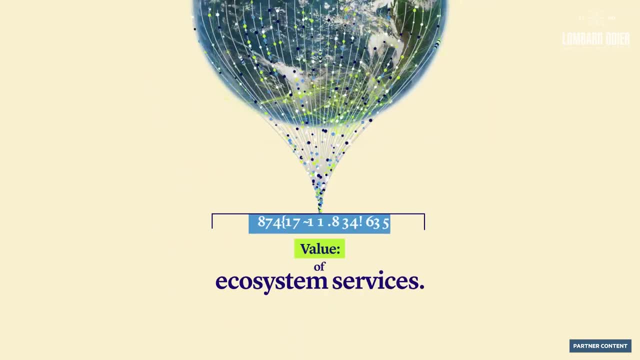 Encaves is a UN-funded research project that is laying the groundwork for environmental and ecosystem accounting With pilots in Brazil, China, Japan, South Africa. the project is laying the groundwork for environmental and ecosystem accounting With pilots in Brazil, China, India, South Africa. the project is laying the groundwork. 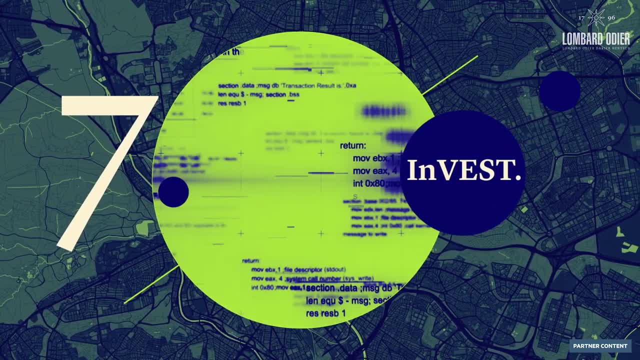 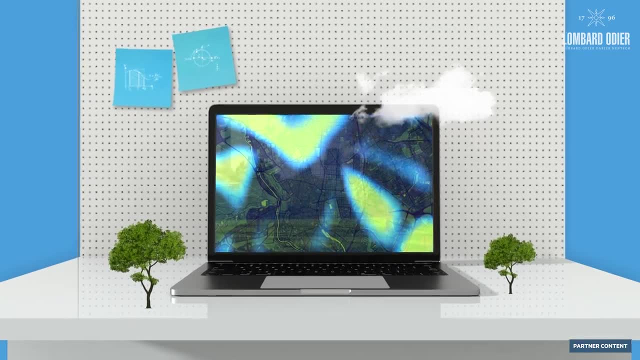 for environmental and ecosystem accounting And two companies are helping to develop new technologies and technologies that make them available to consumers. These tools will help our local businesses to bring in consumers the energy they need for their own problems and their own profits. The software models the links between nature and the wellbeing of populations, demonstrating 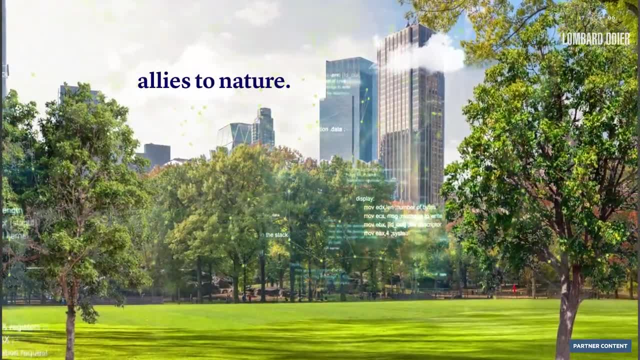 the way investors can become allies to nature. But investing in nature can also mean invest in nature. Here's an example of a new model. In the US, investors are able to increase their income by trading more on natural resources than on iron ore. 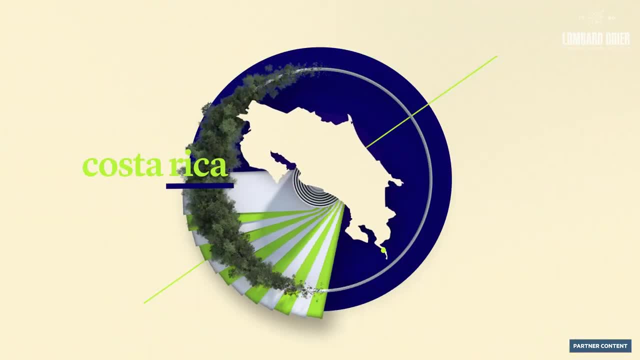 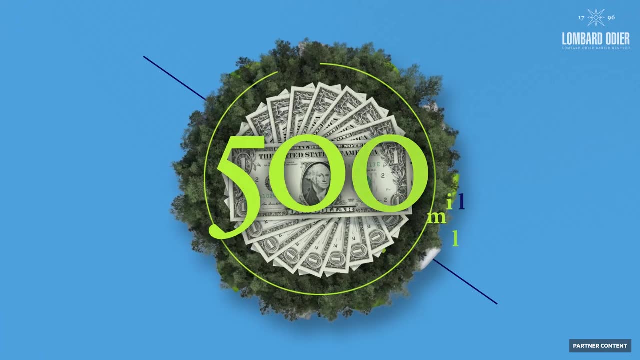 Some so-called industrial products are commonly called industrial products. I'm going to talk about this in just a moment. tropical country to have halted and actually reversed deforestation By taxing fossil fuels. the government has financed a $500 million payout to landowners. 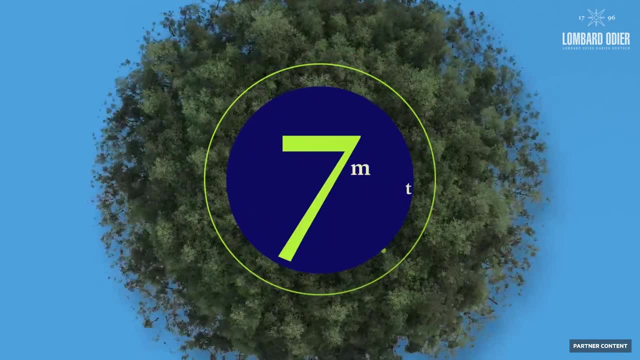 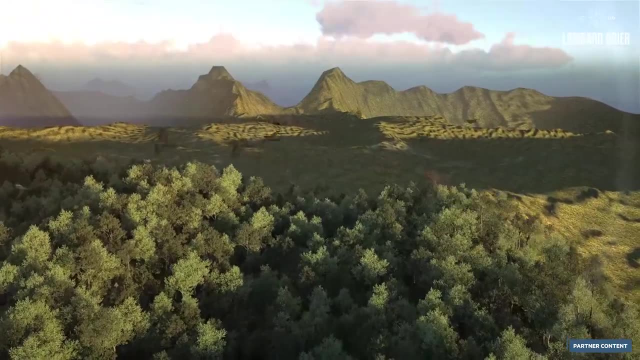 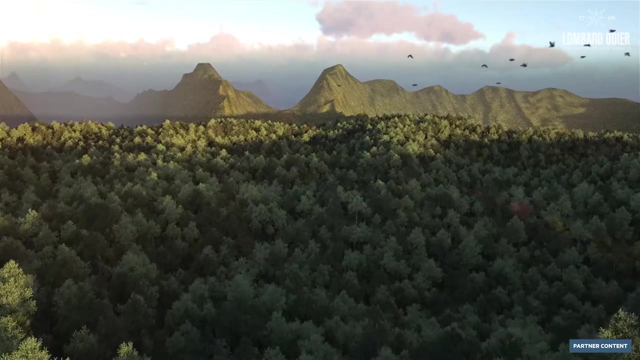 saving more than 1 million hectares of forest and replanting 7 million trees. Whilst many good programs exist around the world, Costa Rica has been recognized as one of the most successful due to political will and a passion for, and recognition of the importance. of their environment.